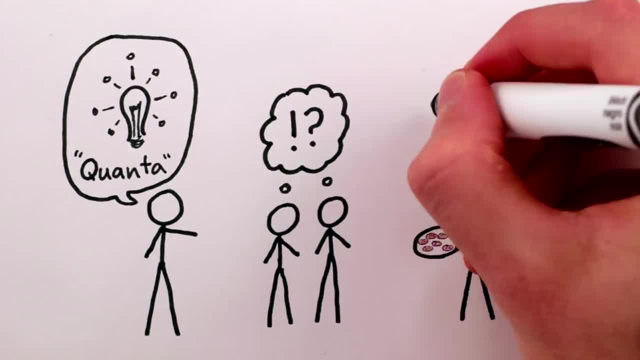 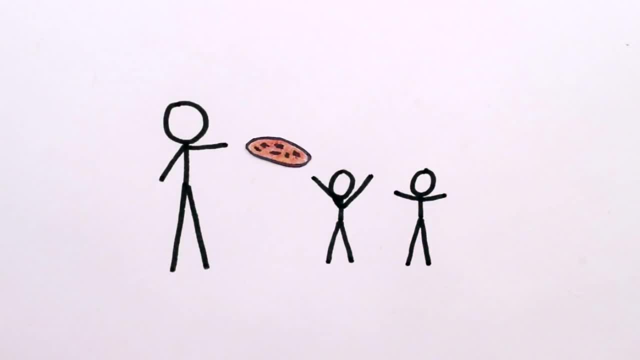 Einstein soon related it to a much more familiar problem: sharing. If you want to make a kid happy, give them a cookie. But if there are two kids and you only have one cookie, you'll only be able to cheer them up half as much. 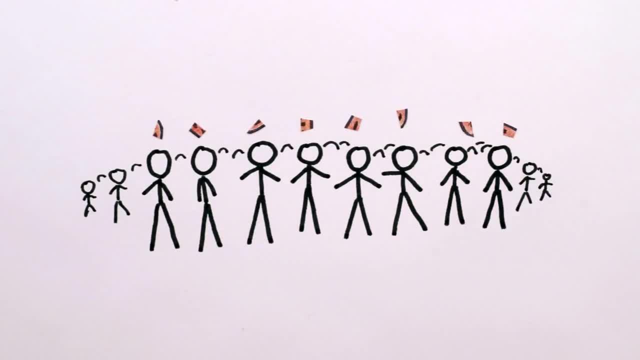 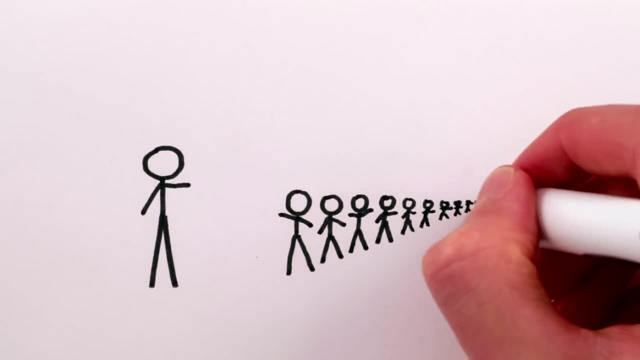 And if there are four or eight or sixteen hundred thousand, you're not going to make them very happy at all if they have to share one cookie between them. In fact, if you have a room with infinitely many kids but not infinitely many cookies, 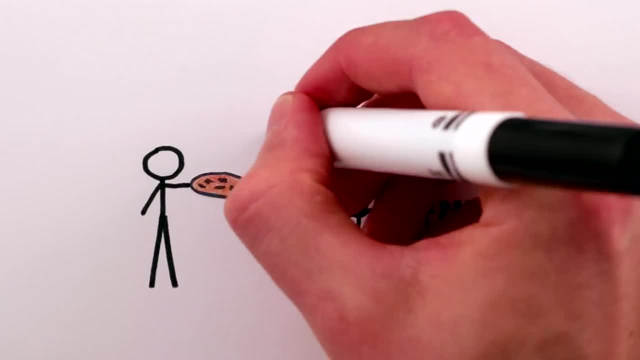 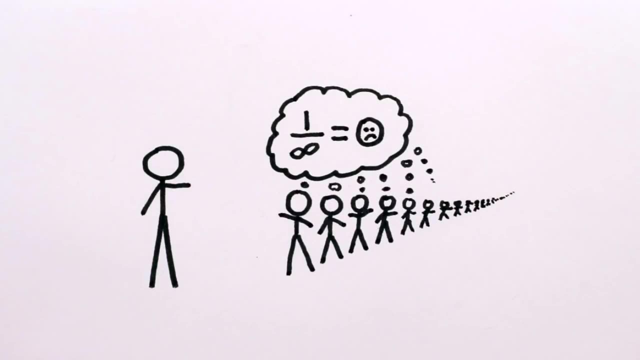 if you share the cookies evenly, each kid will only get an infinitesimally small crumb and none of them will be cheered up, And they'll still eat all your cookies. The difference between light waves and kids is that you can't actually have infinitely. 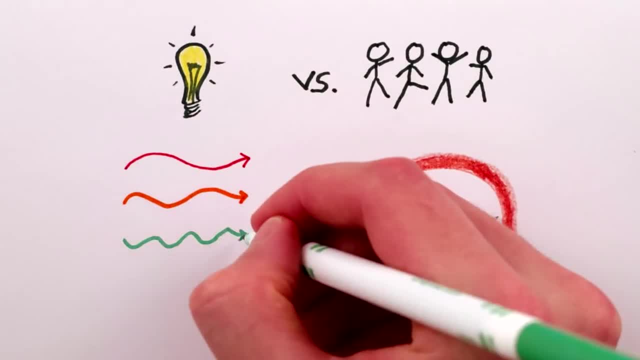 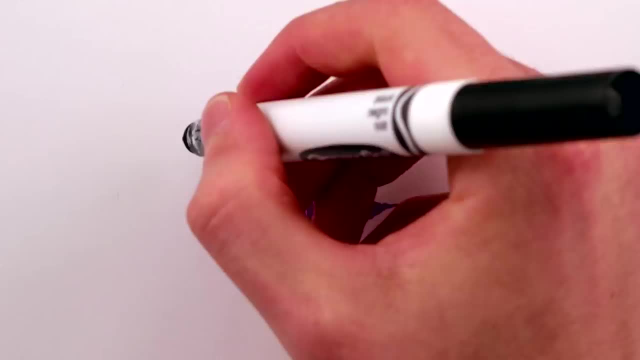 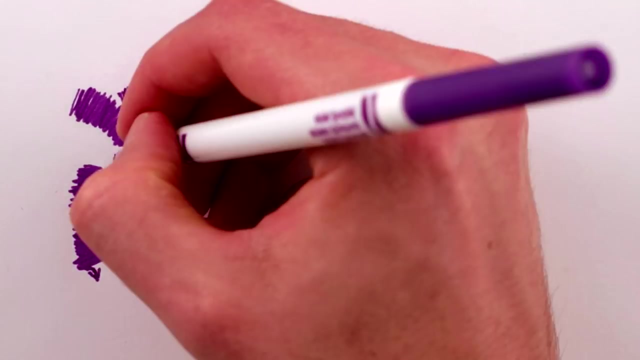 many kids in a room. But because light waves come in all sizes, you can have arbitrarily small light waves so you can fit infinitely many into a room, And then the light waves would consume all your cookies. I mean energy. In fact, all these infinitesimal waves together would have an infinite capacity to absorb. 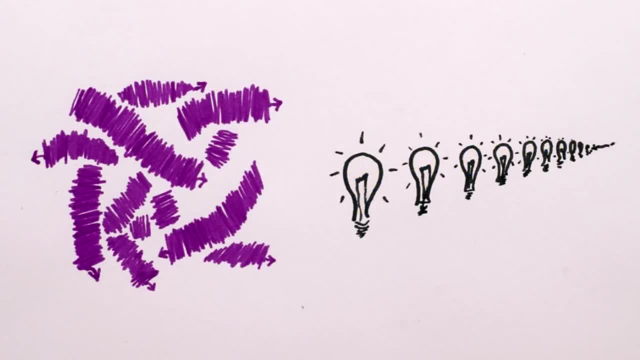 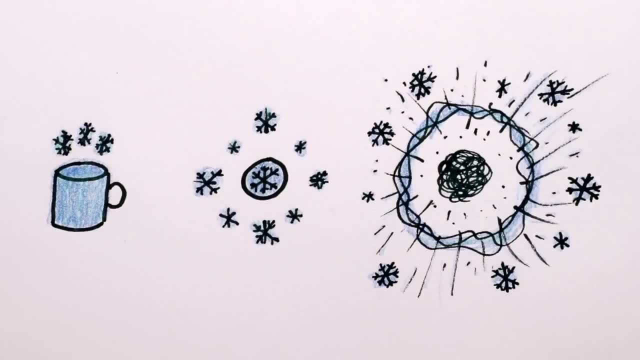 energy And they'd suck all your cookies. They'd draw all the heat out of anything you put in the room, instantly freezing the tea in your cup, or the sun, or even a supernova. Luckily the universe doesn't work that way because, as Planck guessed, the tiny 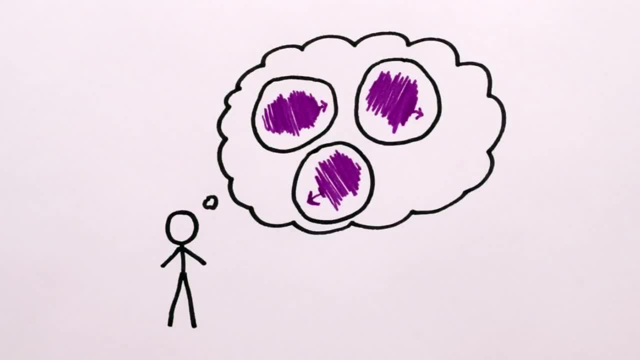 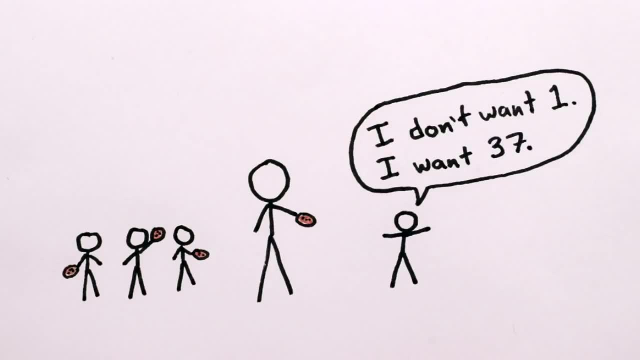 high-frequency waves can only carry away energy in huge packets. They're like fussy kids who'll only accept exactly thirty-seven cookies, or a hundred and sixty-two thousand cookies, no more and no less. Because they're so picky, The high-frequency waves lose out and most of the energy is carried away in lower-frequency. 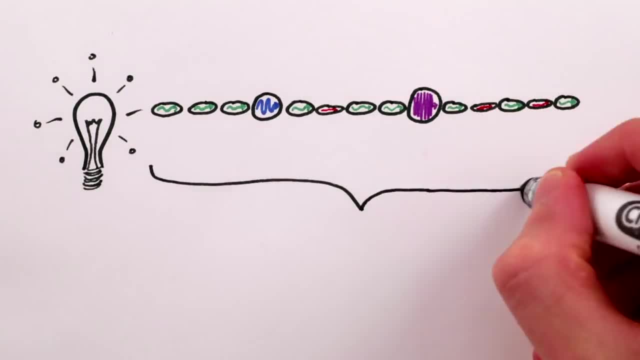 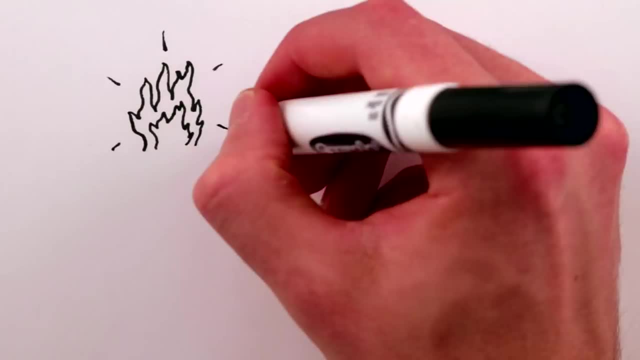 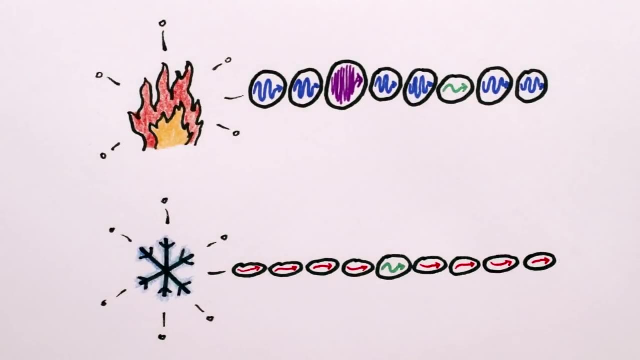 packets that are willing to take an equal share. This common average energy that the packets carry is, in fact, what we mean by temperature. So a higher temperature just means higher average energy and thus, by Planck's rule, a higher frequency of light emitted.